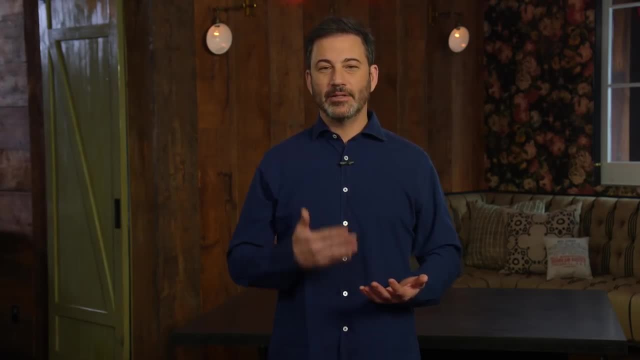 And that man turned out to be Tom Brady, the new quarterback for the Buccaneers. And this is the best part- She kicked him out And look. I know that we need to be safe, and high-profile people have a responsibility to encourage responsible behavior, but I still feel that this is one of the few times it would have been appropriate to say: do you know who I am? 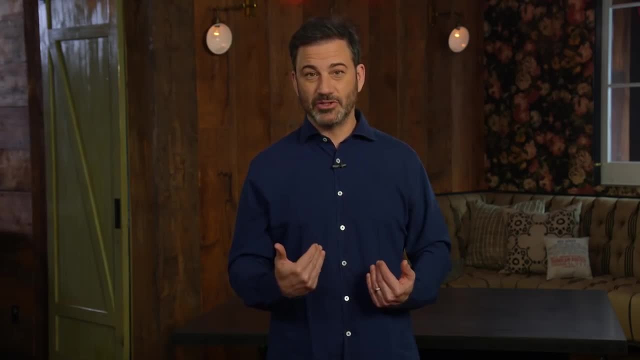 I'm Tom effing Brady. God sent me to win you guys a Super Bowl. You should be staying in your house to keep me safe. Anyway, Tom Brady's at the park working out and his friend Gronk is coming with him. 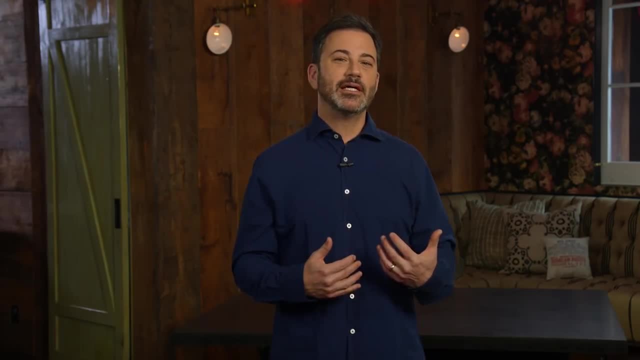 Why, I don't know. Is football even coming back? I have a sneaking suspicion Tom doesn't realize he's living in Florida because he retired last month. A lot of people are working hard during this time, and one group who I feel is not getting enough praise are the people who work at grocery stores. 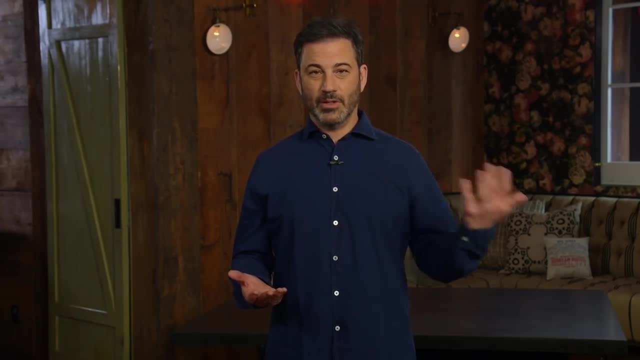 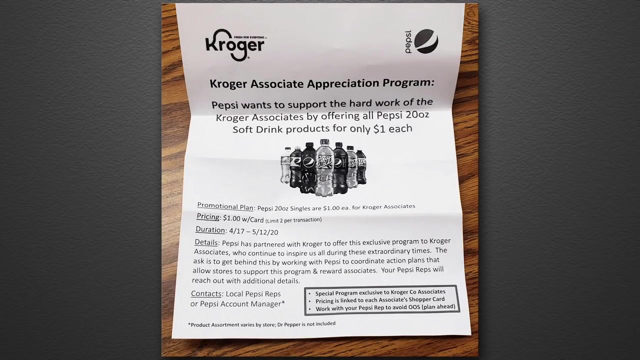 They are putting their health at risk so we can hoard double-stuffed Oreos. But the employees at Kroger in a bunch of cities, did get an incredibly generous From their employer. a flyer was circulated at Kroger that said: as part of their associate appreciation program, to support the hard work of Kroger associates. 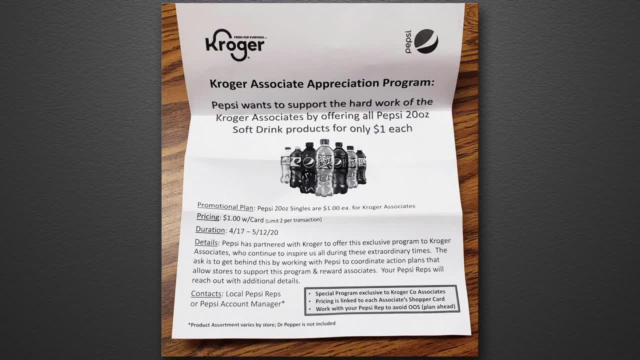 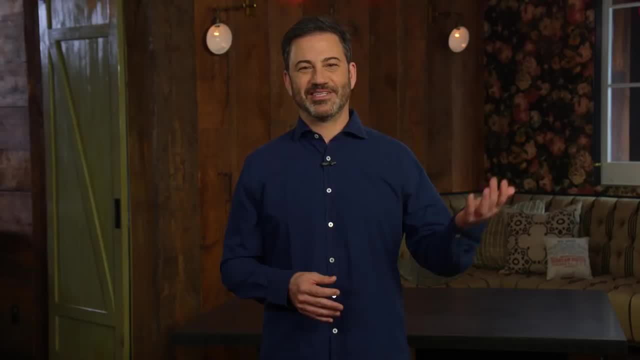 they are offering all Pepsi 20-ounce soft drink products for only $1 each. Limit two per transaction. Dr Pepper not included? Well, of course Dr Pepper isn't included. He's at the hospital right now fighting the virus on the front lines. 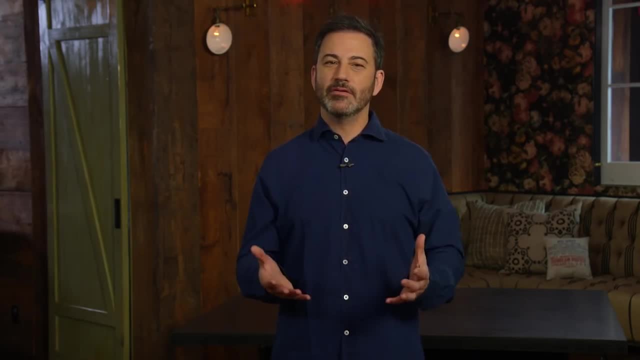 But there you go: More beauty in the face of adversity. Thank you for all you, Mountain Dew. Meanwhile, there are reports that North Korean leader Kim Jong-un is in bad shape health-wise. He is reportedly in grave danger after complications following a heart procedure. 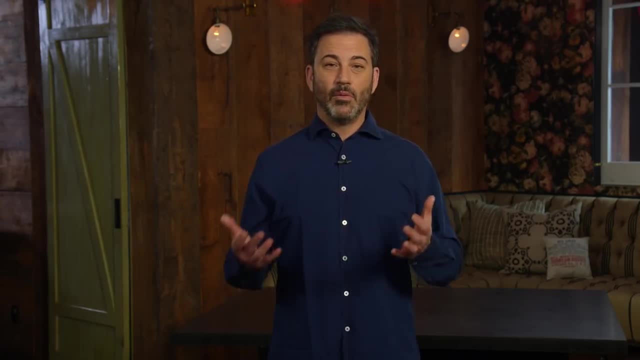 But because everything with him is secretive, no one knows for sure. one of the reasons they suspect he's not well is because last week he missed the most important holiday in North Korea, which is a birthday celebration for his late grandfather, And that's especially alarming. 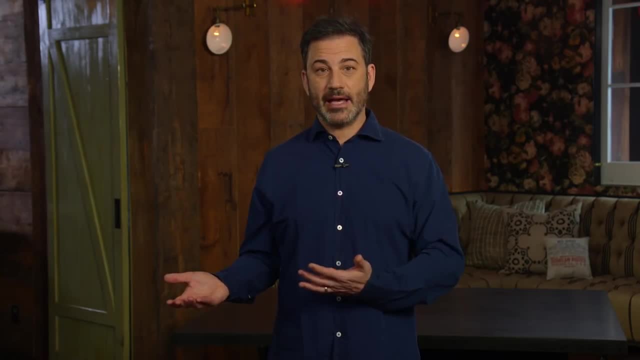 Because you know he is not one to miss the chance to eat cake. A South Korean news site reported that Kim had heart surgery due to complications from excessive smoking, obesity and overwork. See, that's why our president doesn't smoke and never works. 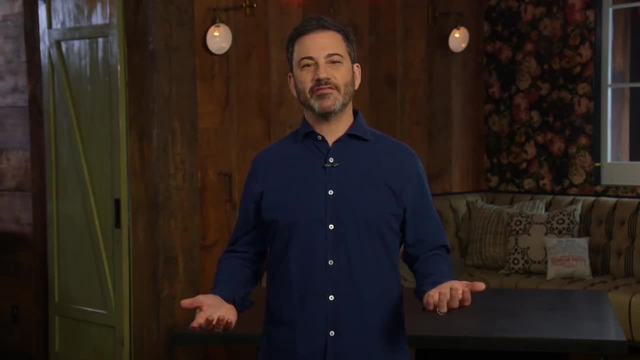 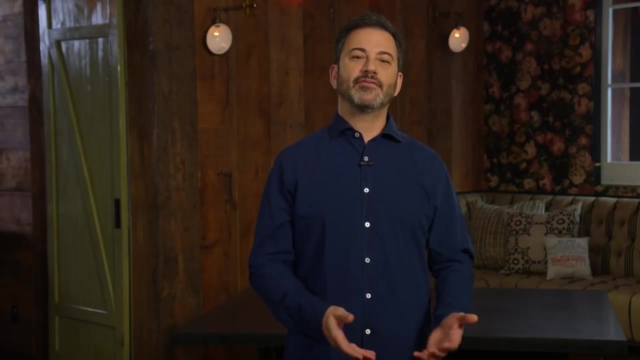 He's smart. Maybe Kim Jong-un just got tired of the whole evil dictator thing and decided to start a new life. He's going to turn up 30 years from now running a bed and breakfast in Vermont, And of course this has to be especially scary. 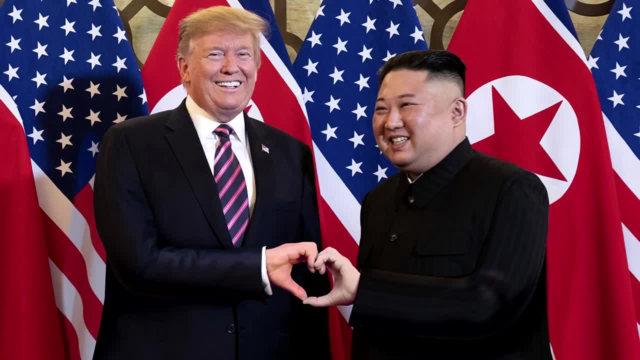 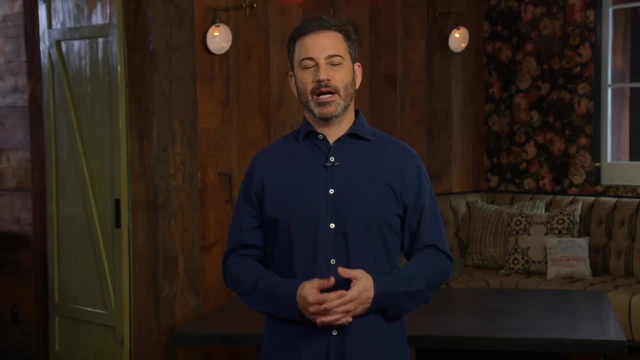 For President Trump, Kim Jong-un is probably his best friend. You know they met many years ago at chubby dictator camp. Trump was up bright and early this morning to remind us that there is an eye in pandemic, and he's it. He tweeted. 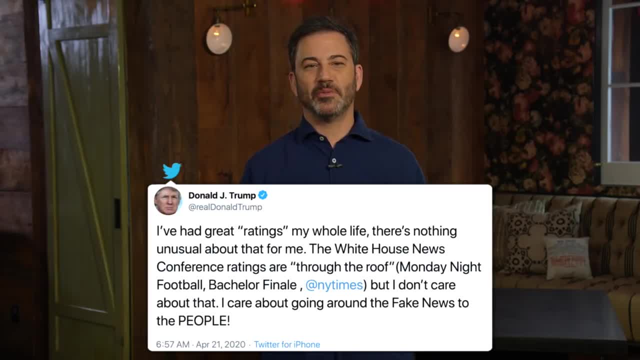 I've had great ratings my whole life. There's nothing unusual about that. for me, The White House news conference ratings are through the roof. Monday Night Football Bachelor finale- New York Times. But I don't care about that. I care about going around the fake news. 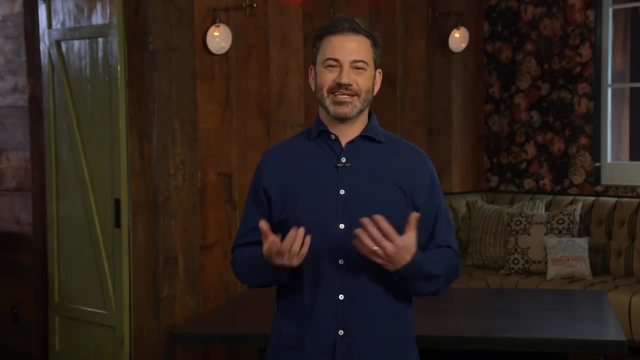 To the people Right. Only Donald Trump would say he doesn't care about ratings, while bragging about his ratings. But it wasn't all lashing out. In fairness, Trump did try to lift spirits yesterday and actually told a pretty funny joke. 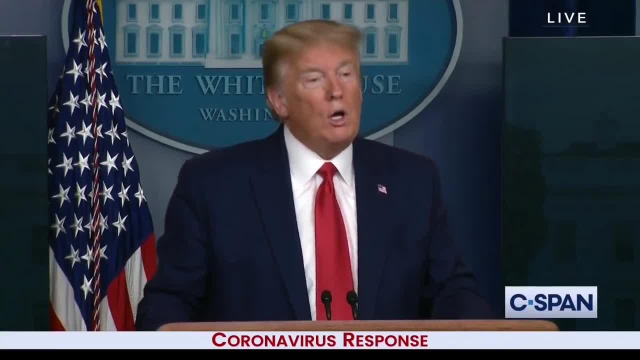 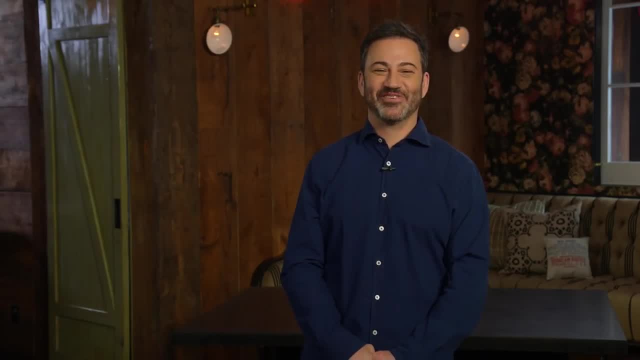 Please go ahead. No, I think right behind you. I promised I can't. I cannot tell a lie, So we'll get you next. OK, It's a good one. And guess what? He didn't get her next. 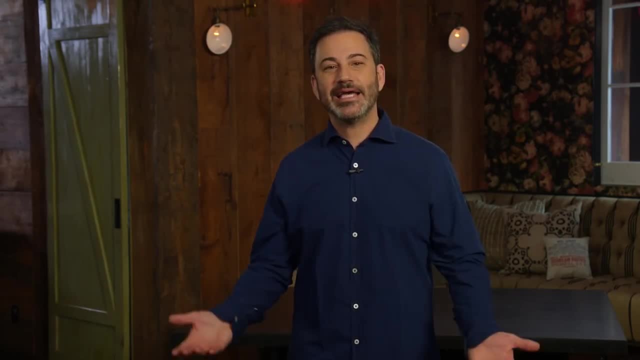 He went to someone else And then, Moments later, he lied again. You held rallies in February and in March And there are some Americans. Oh, I don't know, I don't know about rallies, I really don't know about rallies. 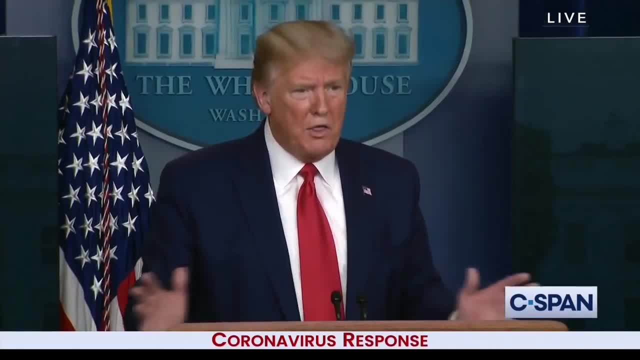 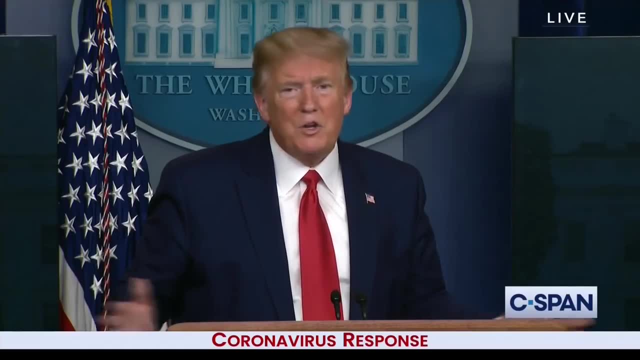 I know one thing: I haven't left the White House in months, except for a brief moment to give a wonderful ship the comfort. You held a rally in March. I don't know, Did I hold a rally? I'm sorry, I hold a rally. 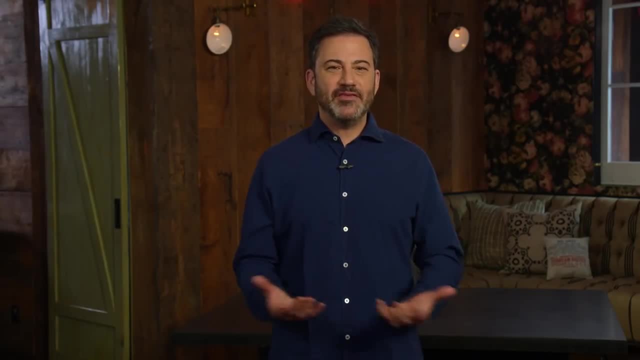 Did I hold a rally? Did I hold a rally in an enclosed space, even though I now claim to have known it was dangerous at that time? Yes, Do I have an advent calendar counting down the days until I can hold my next one? 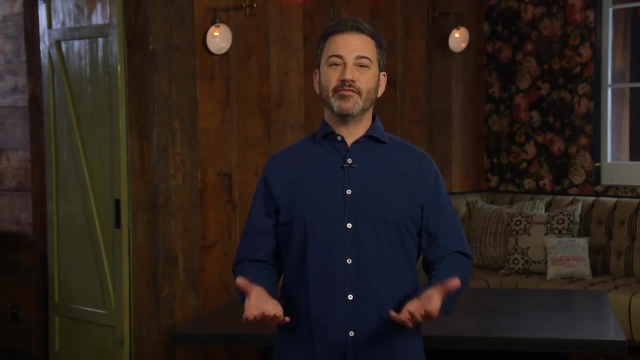 You bet your dirty mask, I do. He held rallies in February and March And he left the White House four times in March, including a trip to Mar-a-Lago. Mar-a-Lago, by the way, laid off 153 workers today, in addition to the 560 laid off at Trump's resort in Miami. 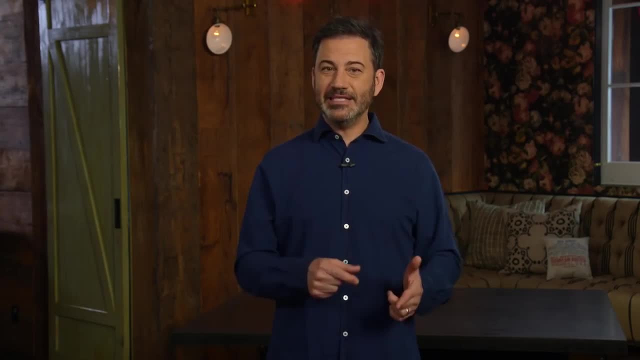 Maybe this is why he's so anxious to open for business again. He's getting hurt. This gives you a sense of how things are going at the White House. Yes, The president's own coronavirus task force- members of his own team are reported to be actively ignoring him now. 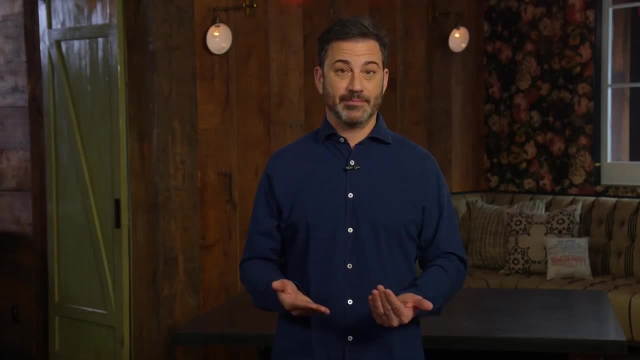 They say the vice poodle, Mike Pence, won't even sniff his butt, which I don't know. That doesn't make any sense to me. Why would they ignore a president who has so many great ideas? Remember when he wanted to nuke the hurricane? 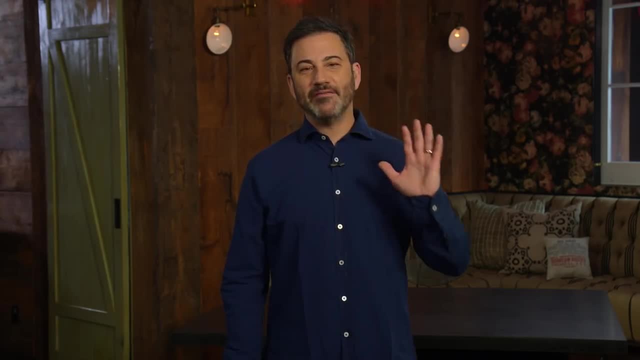 You probably think I'm joking, but go ahead and Google that. I have a lot of questions about the president's task force and the mixed messages we've been getting about staying home. So we reached out to the White House And, believe it or not, they connected us with the chief medical advisor to the coronavirus response team. 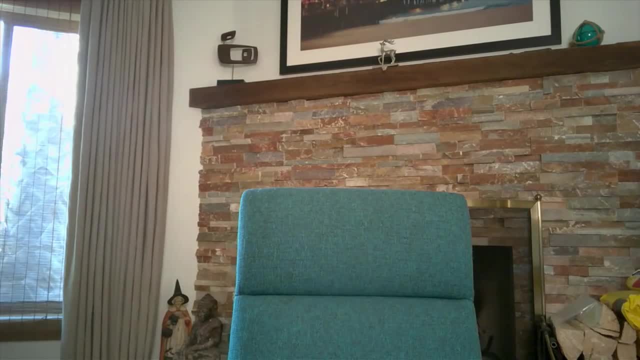 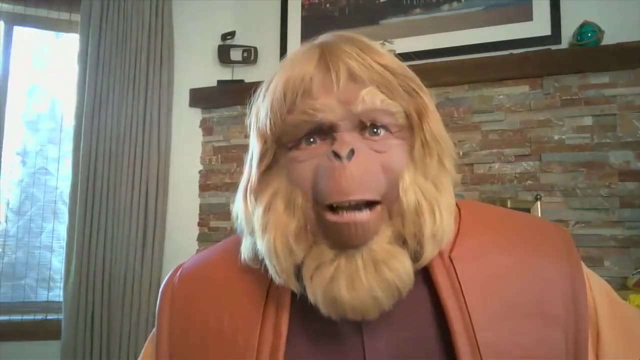 And I am honored to welcome Dr Anthony Fauci. Hello, Dr Fauci, Dr Fauci, Hello, Hello. Can you hear me on this? Hello, Yes, yes, we can hear you, But I was under the impression I'd be speaking to Dr Fauci. 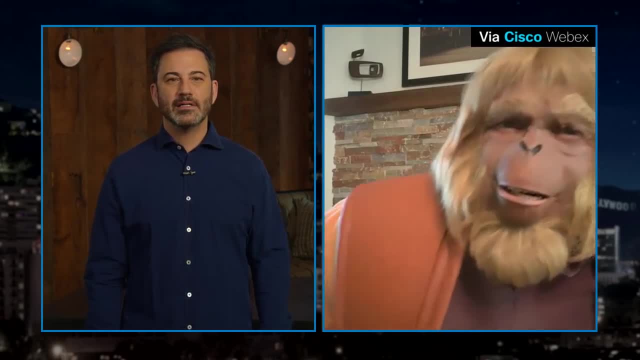 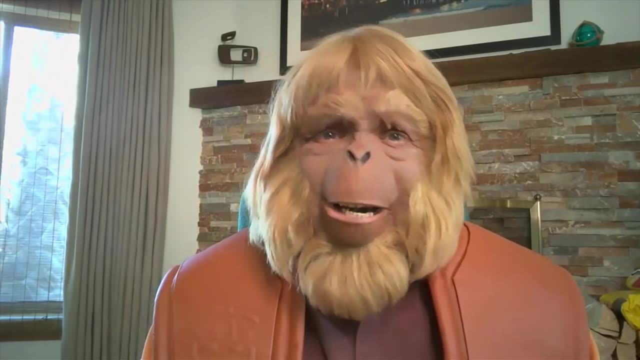 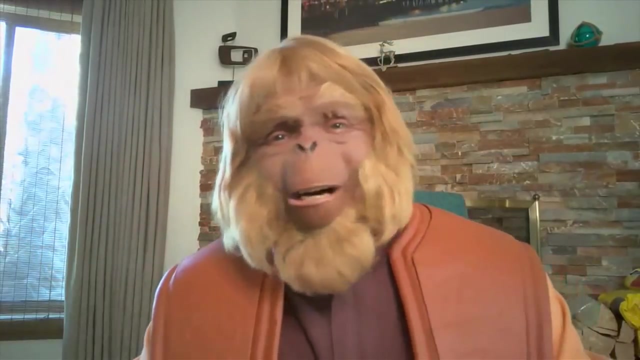 Oh, no, no, Dr Fauci is no longer with us. Why, Why, What? Well now, the president respects disagreement And he respects Dr Fauci so much that he actually sent him to a big farm upstate where he's free to run around in a field all day with other doctors. 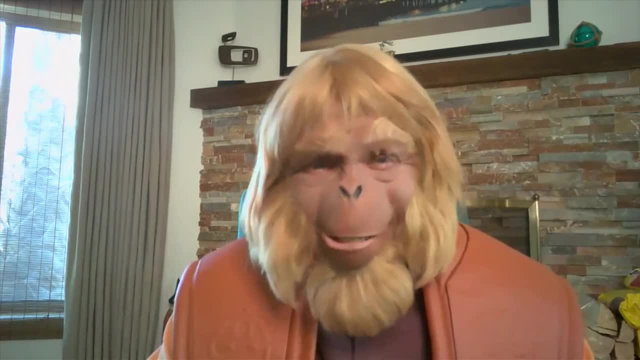 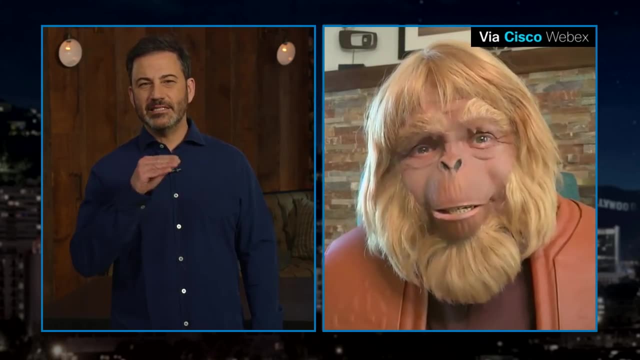 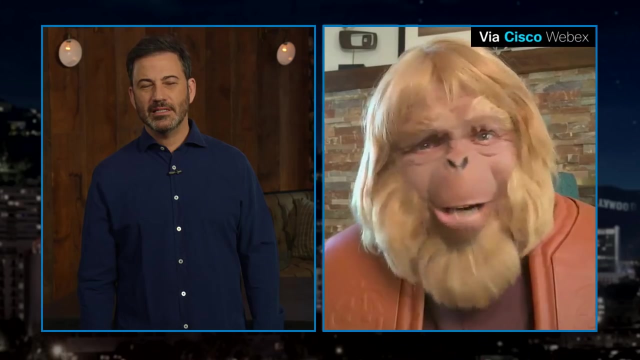 I'm the new lead on the coronavirus task force And you are, Oh, Dr Solomon Zayas, As in Dr Zayas, the diabolical minister of science from Planet of the Apes. I've done other movies, Oh, okay. 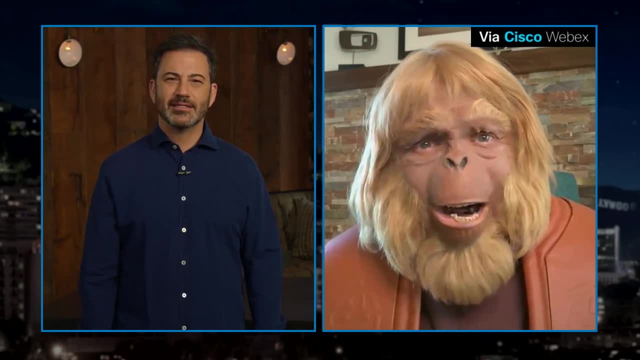 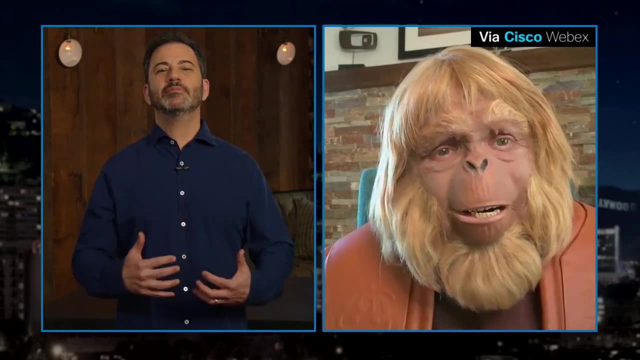 Well, Dr Zayas, what other movies have you done? A little thing called Jumanji, Maybe you've heard of it. Yes, All right. Anyway, Dr Zayas, if you don't mind me asking, how did you get this job? 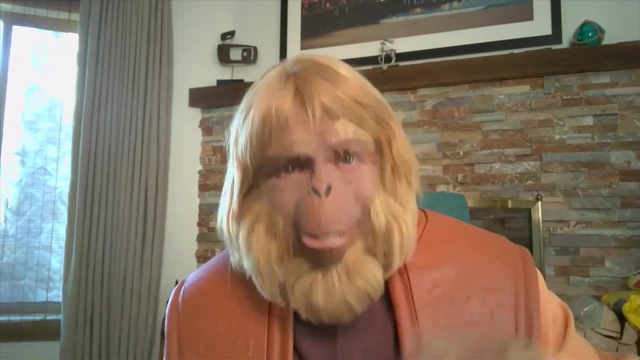 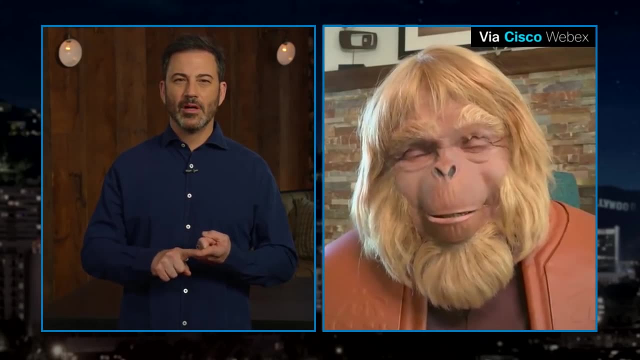 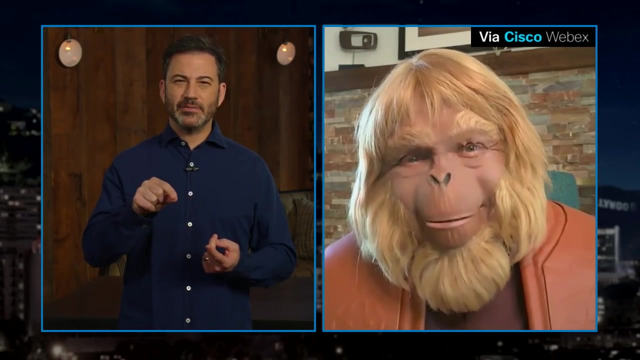 Oh, family connection. The president's mother Mary is my nana's sister, Okay, Okay, so your mother Was his mother's sister, But you're in An orangutan. yes, Wait, so that means Donald Trump is.